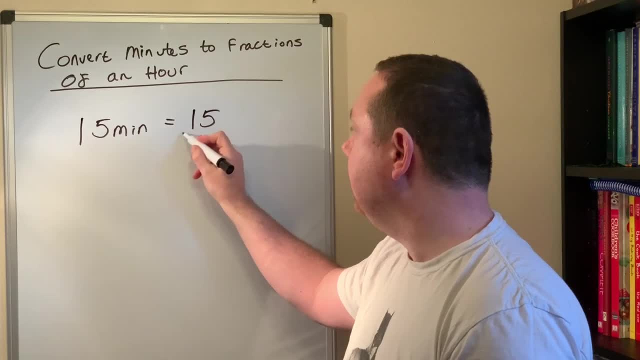 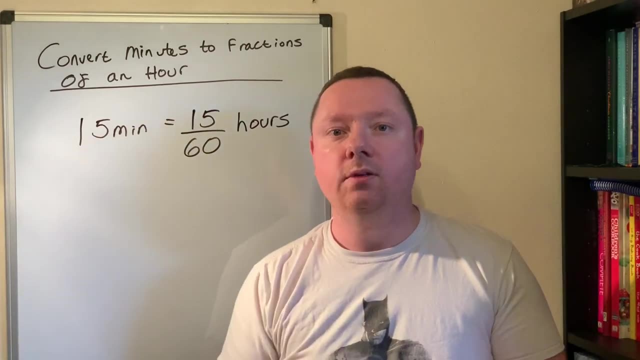 first thing I would always do is do 15, that's out of 60.. It's as simple as that. it's 15 out of 60.. hours Now. we don't want to always have to work with a fraction like 15 out of 60, especially if 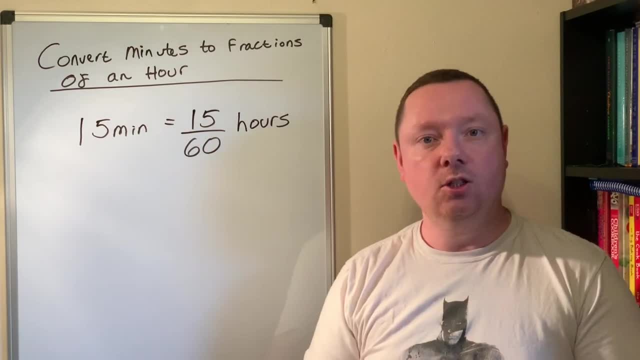 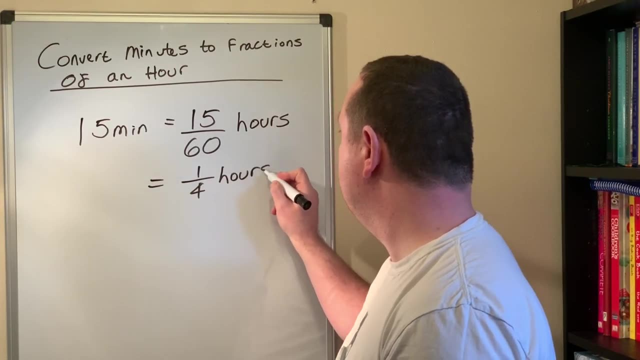 we're not using a calculator, so we always try and simplify our fractions as best we can. 15 out of 60 is a quarter, so that's a quarter hours, or if we were doing that as a decimal, we should all know that quarter is 0.25.. 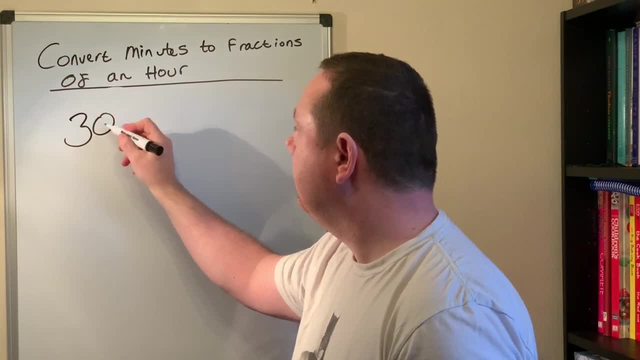 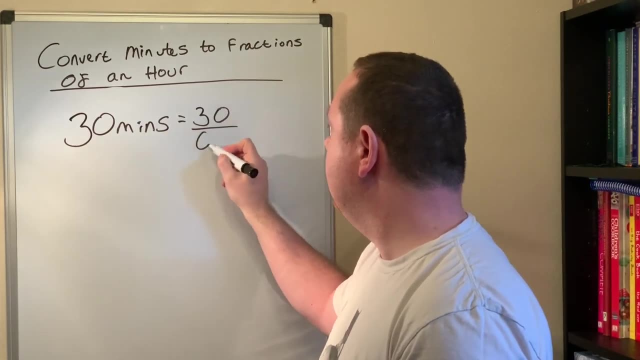 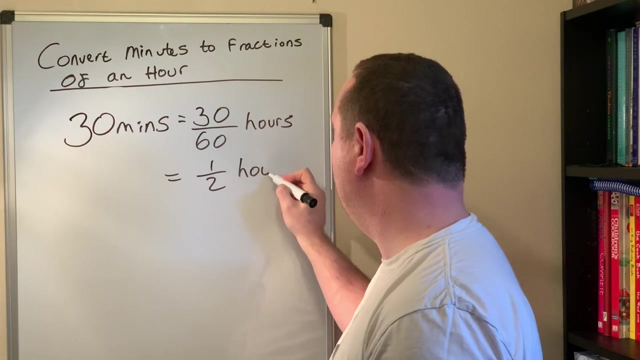 Let's do another simple example, classic one: 30 minutes. we all know that's half an hour. but if we didn't do 30 out of 60 hours, simplifying that 30 out of 60 is a half hour or 0.5. I've got 12 minutes. 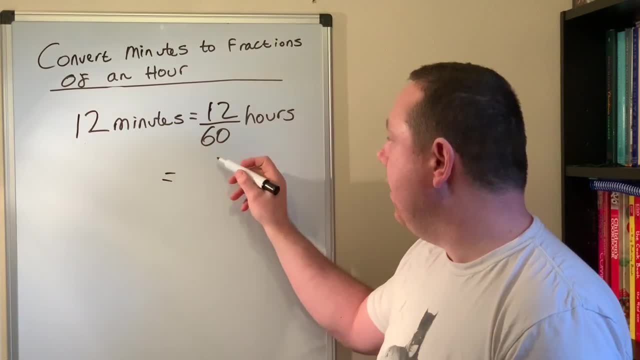 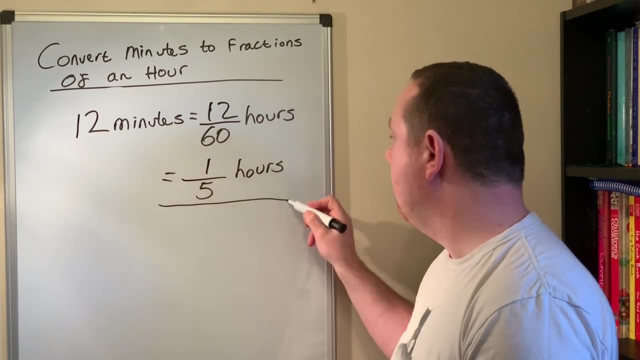 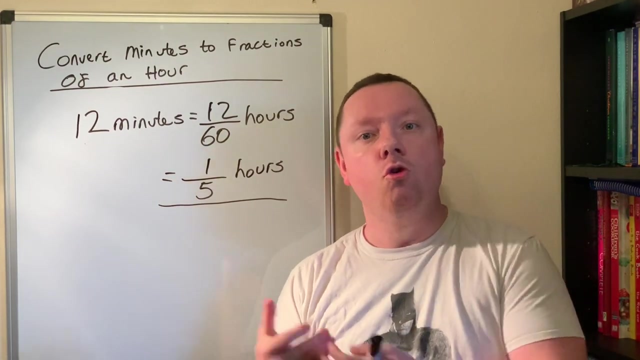 that's 12 out of 60 hours, so I can divide the top and bottom by 12 to get one out of five, a fifth hours Okay. so hopefully that gives you a very simple overview of how you can be at minutes. two fraction of an hour, okay, and we're going to use that in a few simple problems using speed to 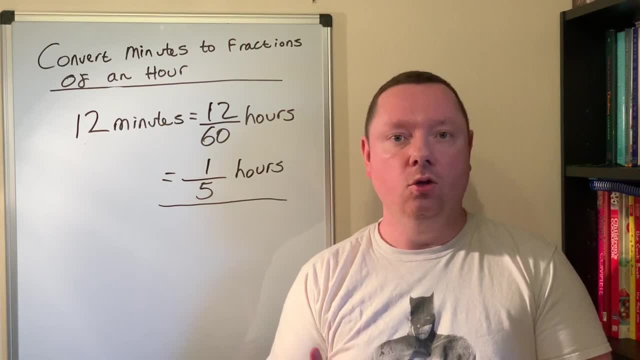 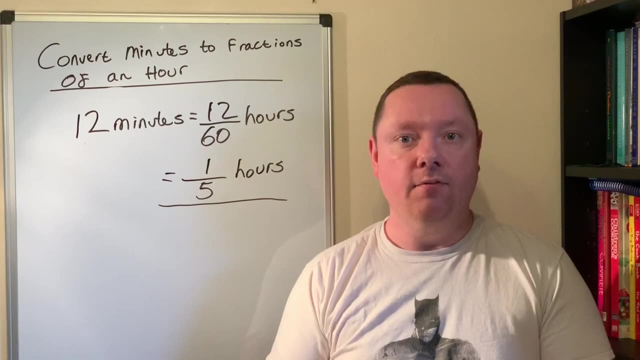 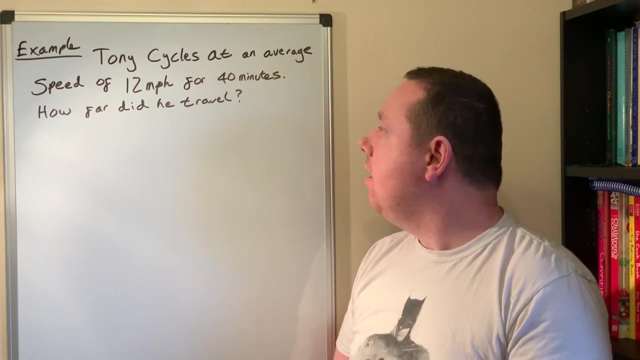 distance time, which you should all really know how to do because of the previous video which overviewed how to use the speed to distance time formula. If you're not sure how to do that, please check that video out. Okay, example: Tony cycles at an average speed of 12 miles per hour. 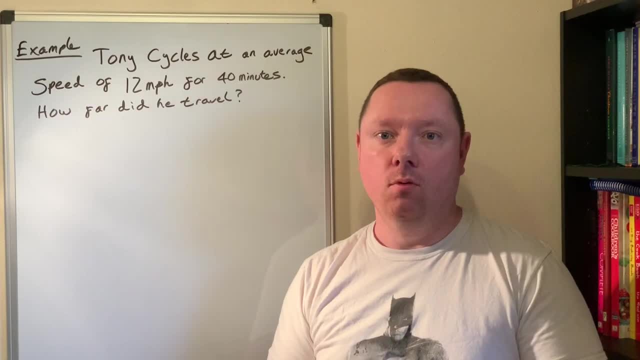 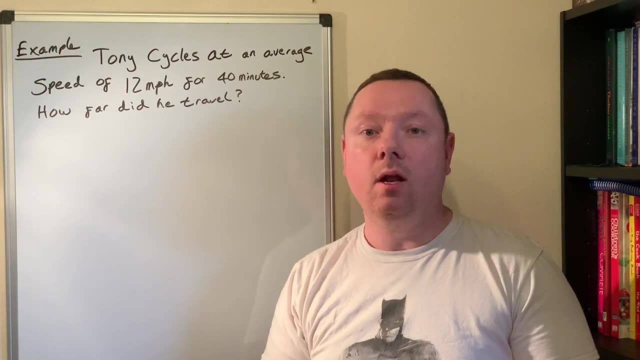 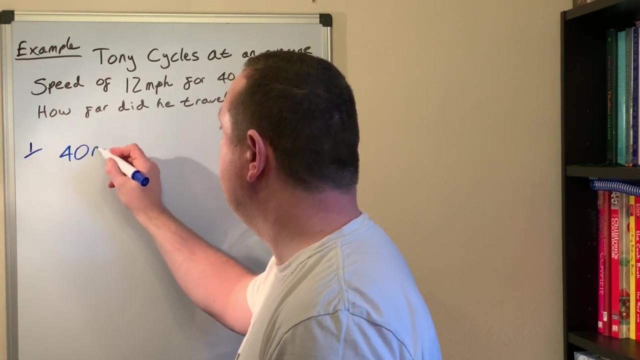 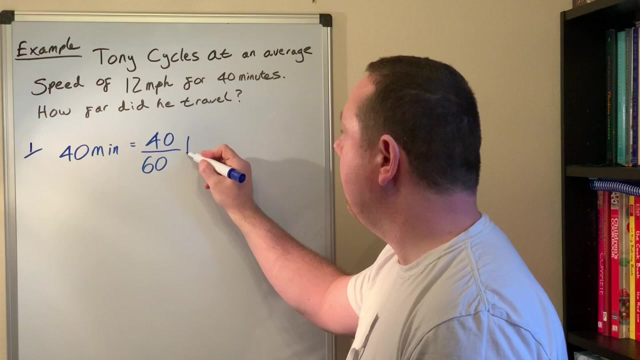 for 40 minutes. How far did he travel? Step one is to always check our units. Hours, miles per hour, minutes- these are completely different, so how do I have to compare my minutes to hours? So step one: 40 minutes equals 40 out of 60 hours, always out of 60.. 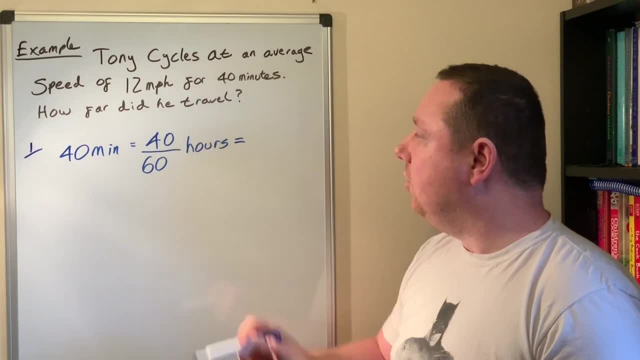 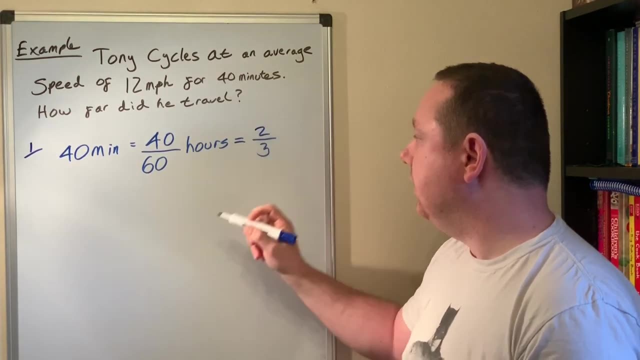 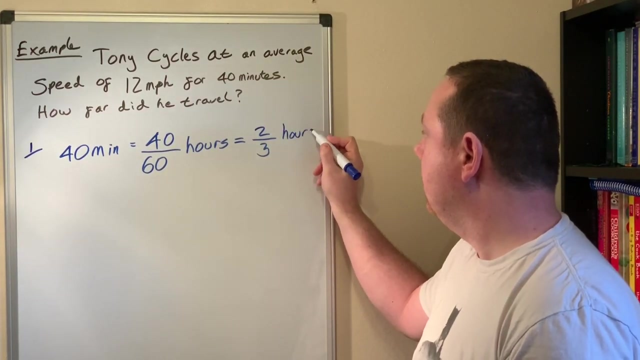 Simplifying my fraction. I can divide the top and bottom so I get two thirds hours. That's simply dividing by 20 to get two and by 20 to get three, so I get two thirds hours. Step two is exactly the same as when it's just a standard speed distance time. 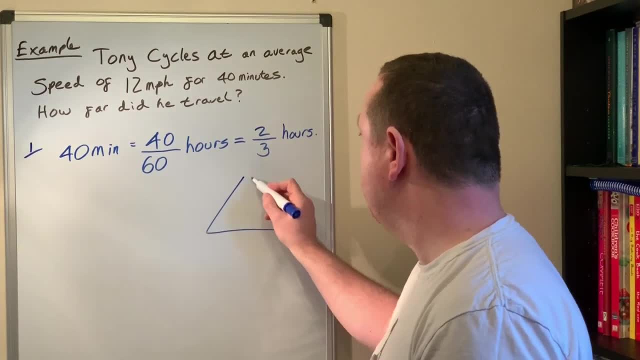 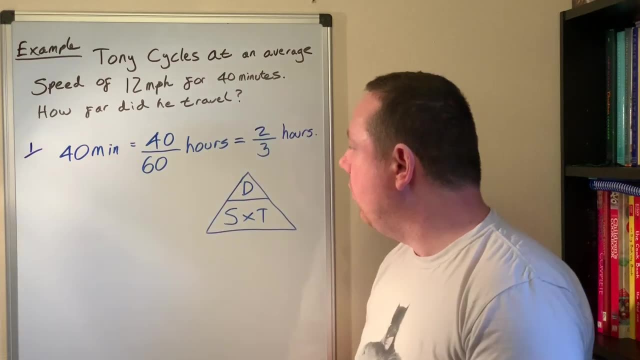 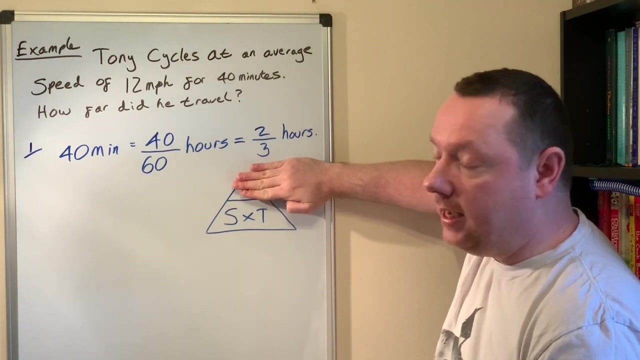 problem. We draw our speed distance time triangle- remember distance at the top over speed times time. I cover up the one. I want distance in this case because it's how far I traveled. So it tells me straight away that distance is speed times time. So step two: I write down distance. 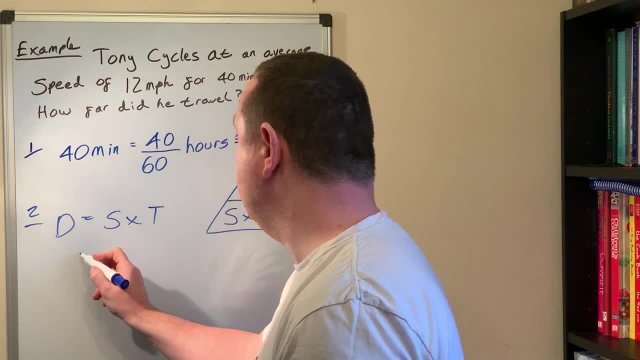 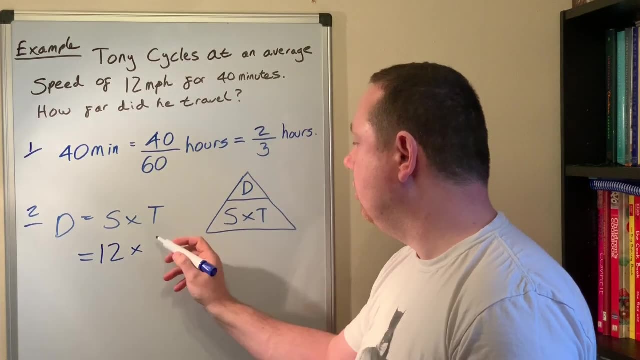 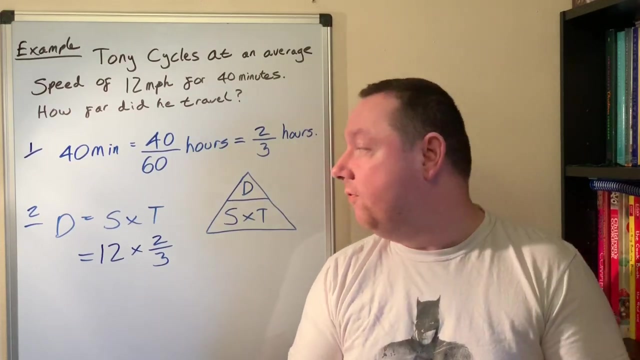 equals speed times time and I substitute in what I've got, 12 miles per hour times my new time, which is two thirds over an hour Times and by a fraction is the same as doing a fraction over an amount. A quick reminder of that: it means you times by the top and divide by the bottom, So 12 times 2 is 2.. 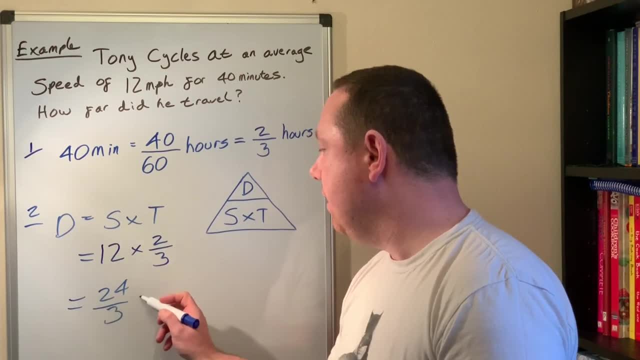 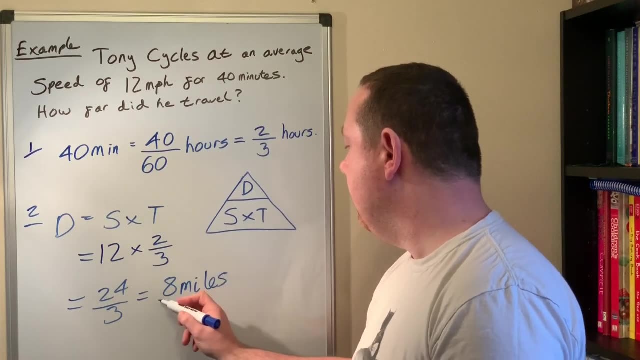 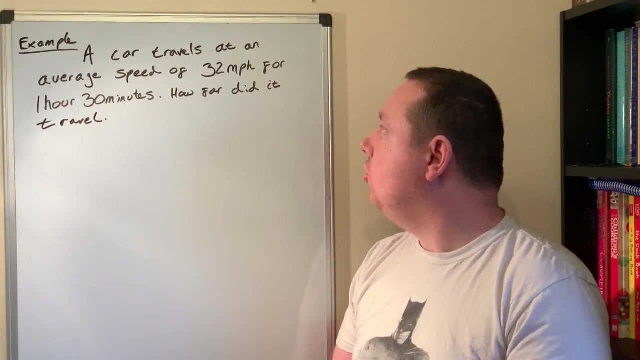 24 divided by 3, which is 8.. And the units will be miles, because it was miles per hour. So the answer we get is 8 miles. Okay, example two: This car travels at an average speed of 32 miles per hour for one hour and 30 minutes. How far did it travel? So again, we've got a mixture of 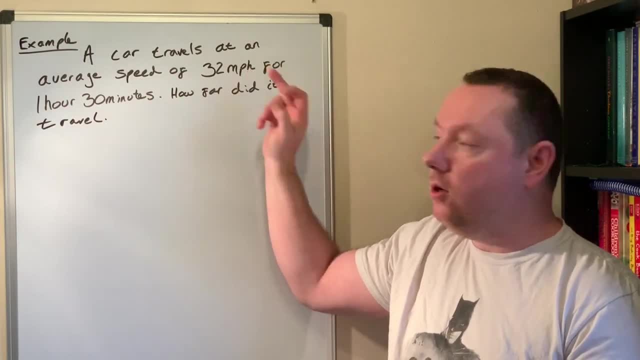 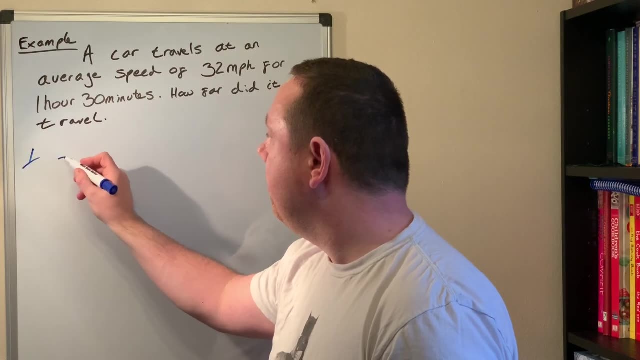 hours and minutes here this time and we've got hours and our miles per hour. so we're going to have to convert this into one whole fraction. So we'll take the minute part first. 30 minutes. Well, that's 30 out of 60. 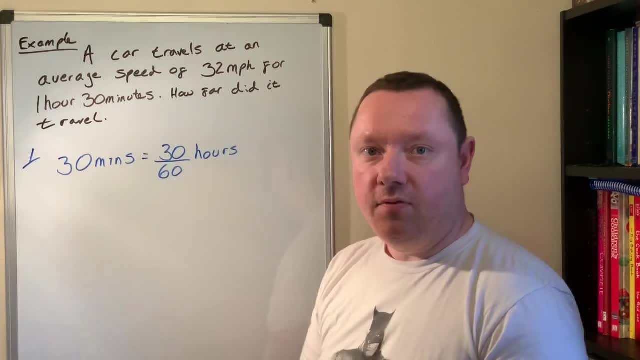 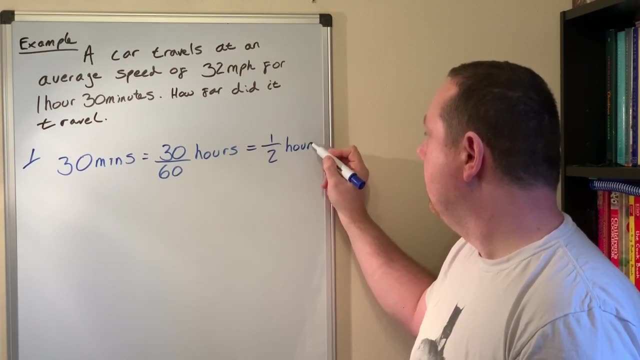 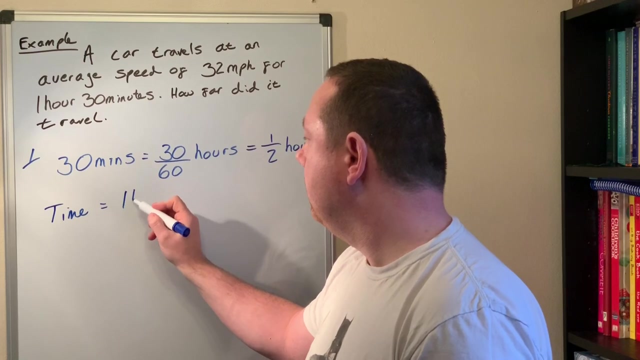 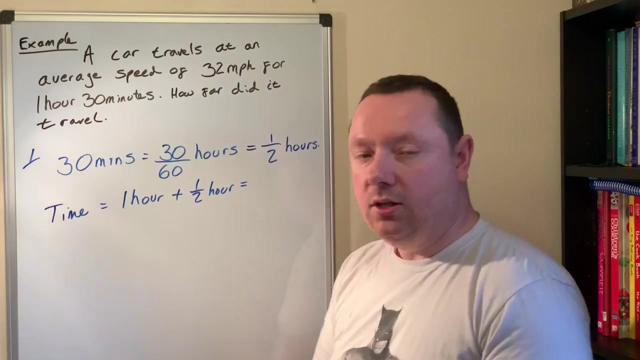 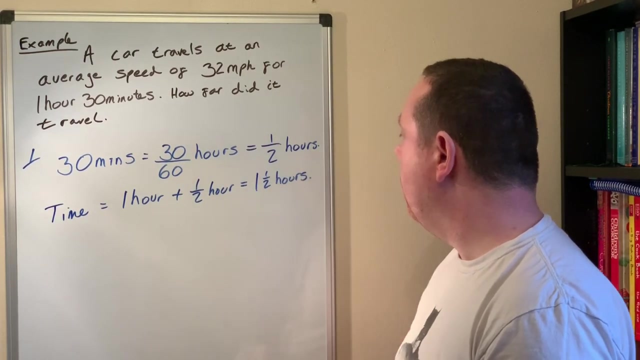 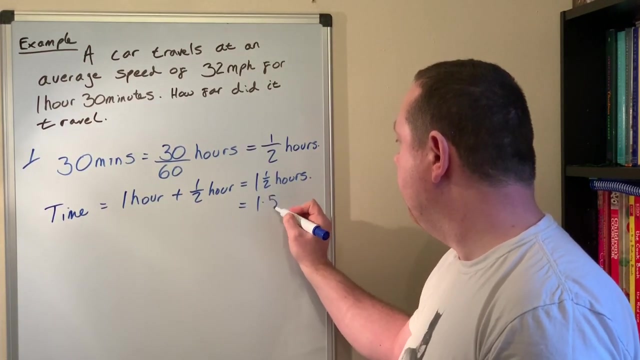 hours, which we can simplify quite easily by dividing by 30 on top and bottom, to get one out of two a half hour. So our total time is going to be one hour plus a half hour. Well, that's one and a half hours, which, for this video, I'm going to change to 1.5 hours, because a half is 0.5.